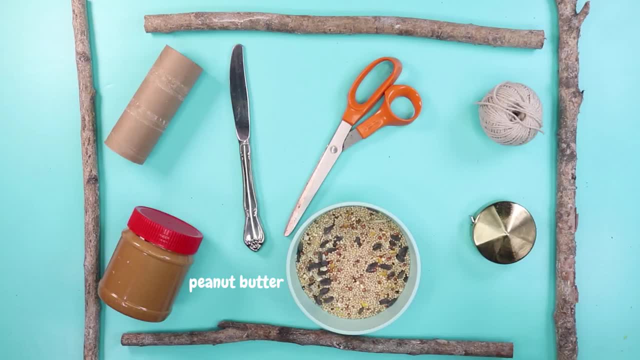 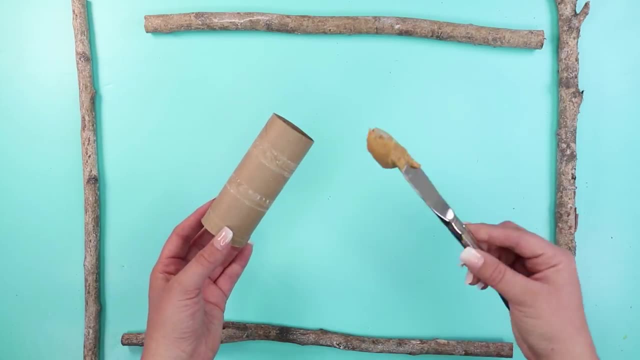 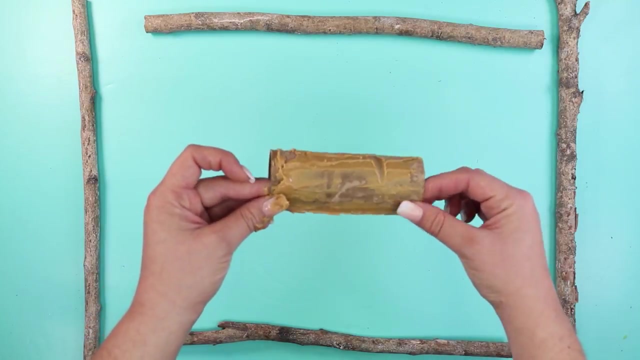 For the first one, you will need a toilet paper roll, peanut butter, a butter knife, scissors, bird seeds, measuring tape and a string. Begin by spreading delicious peanut butter on the toilet paper roll with a butter knife. Next roll your toilet paper roll against the 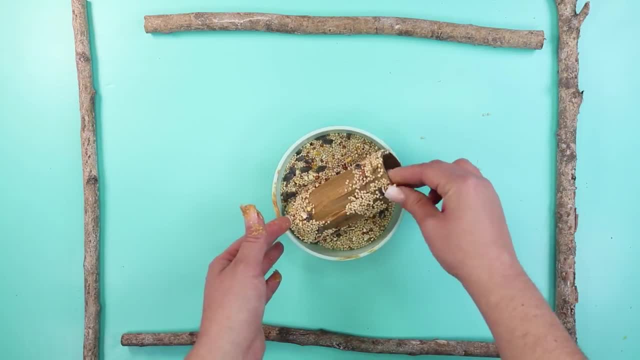 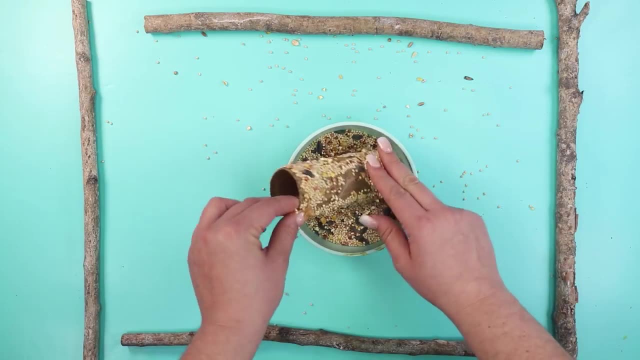 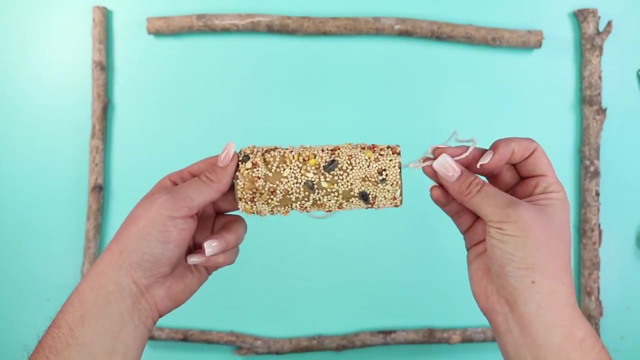 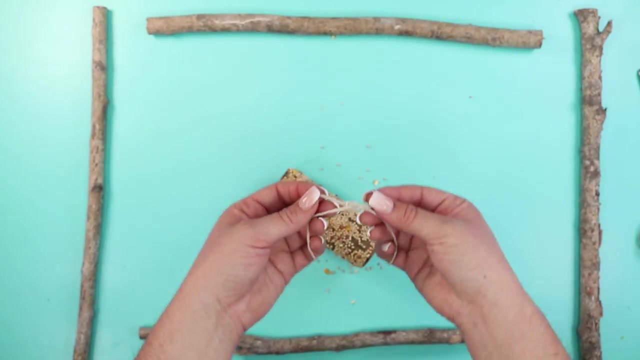 seeds so that they stick until the entire thing is covered. It's okay to get a little messy. Measure 25 inches on your measuring tape to measure the length of the string and cut. Pull your string through the middle of your roll, tie a knot and voila, Now hang your bird feeder. 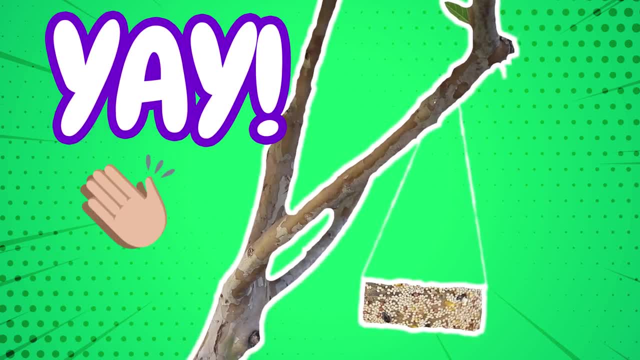 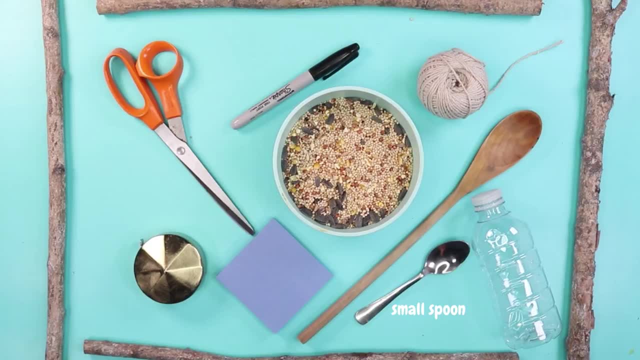 on a tree branch. Yay, The spinning around feeder. For the last fun bird feeder of the day, you will need a plastic bottle, a small spoon, a wooden spoon, string bird seeds, a sharpie wood, post-it scissors and a measuring tape. First, draw a circle on the bottle near the 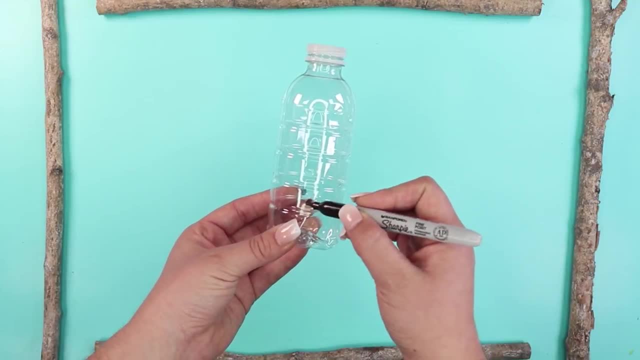 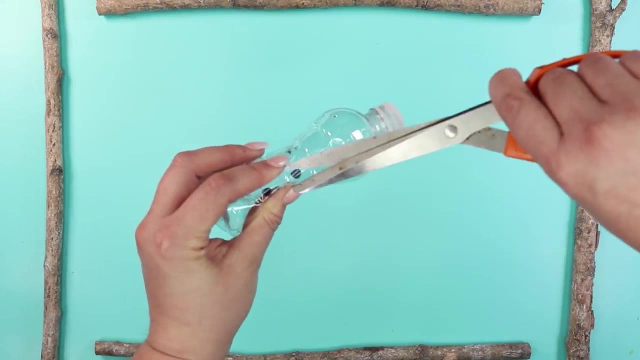 bottom about the size of your wooden spoon's end. Flip your bottle to the other side and draw a circle directly across the one you made. Draw a third circle an inch above that one. Ask a grown up to help you cut out those three holes. Now slide your wooden spoon through the two lower. 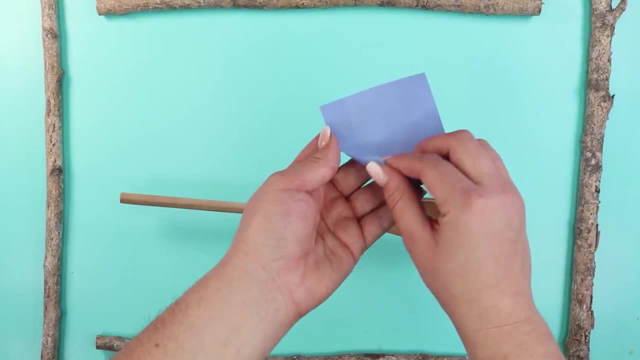 holes. That sure is a sturdy perch you've made With your post-it note. make a cylinder-shaped funnel and fill the funnel For the second one. make a cylinder-shaped funnel and fill the funnel For the third one. make a cylinder-shaped funnel and fill the funnel For the fourth one. make a cylinder-shaped. funnel and fill the funnel. For the fifth one, make a cylinder-shaped funnel and fill the funnel. And make another cylinder-shaped funnel For the fourth one. make another cylinder-shaped funnel. For the fifth one, make a cylinder-shaped funnel and fill the funnel. 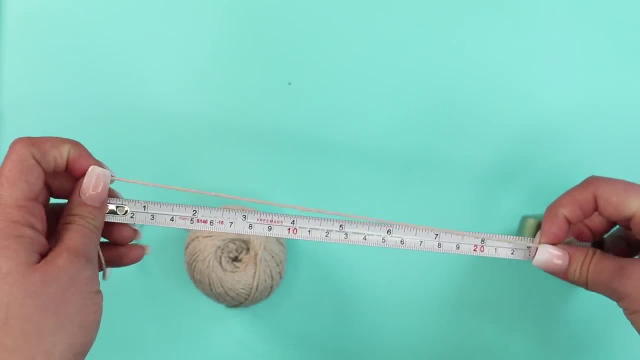 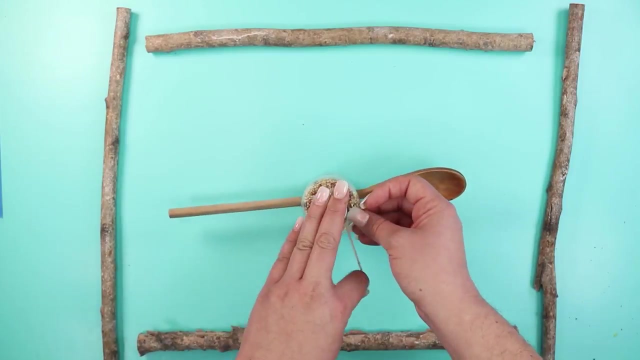 Now make a feeder. to make a bigger feeder hole. For the fifth one, make a feeder hole. Measure nine inches of your measuring tape to measure the length of the string and cut. Tie one knot around the bottle's opening rim And another one to make a hole. 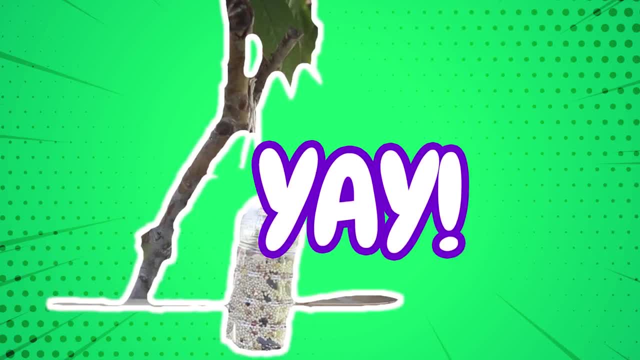 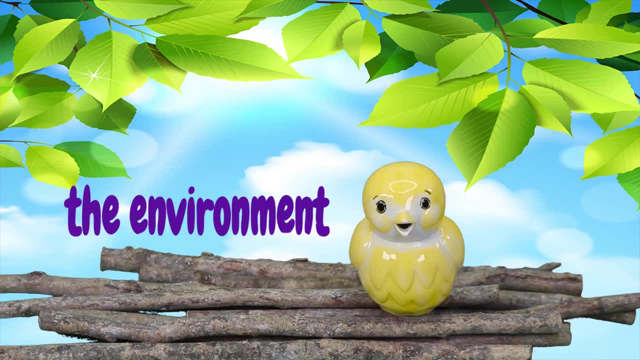 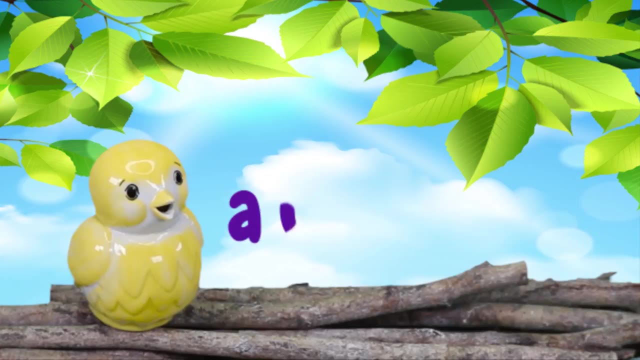 Now it's ready to hang outside. Yay. By recycling your leftover stuff and turning it into bird feeders, you're helping the environment and giving my friends and i a meal. thanks for making bird feeders with me. make sure to click the red button to become a unilander. 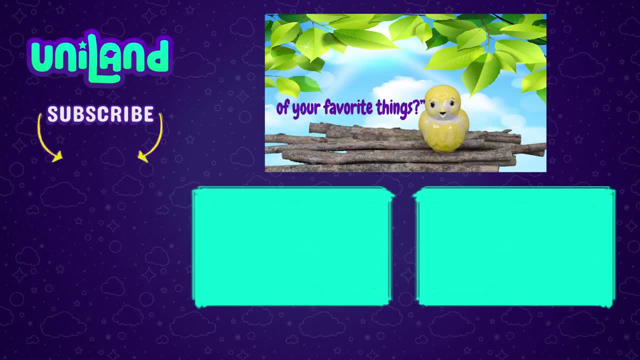 what are a few of your favorite things? let us know in the comments down below.